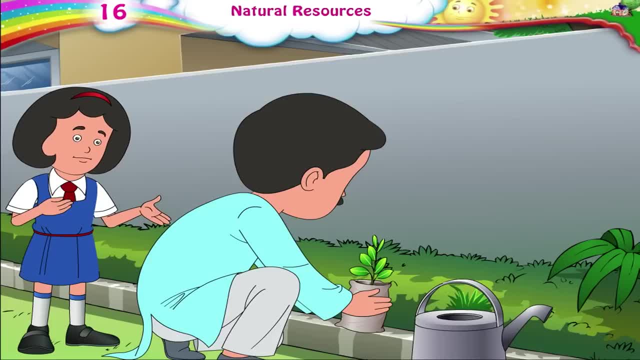 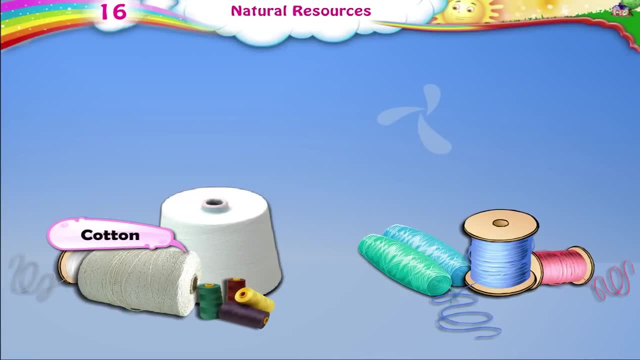 Paper, rubber and colours are all got from trees, Even our clothes, papa Remember we learned about fibres: Carbon, Cotton And other fibres. comic books, функ, Leader Of letters, Punk Timing. toast to. 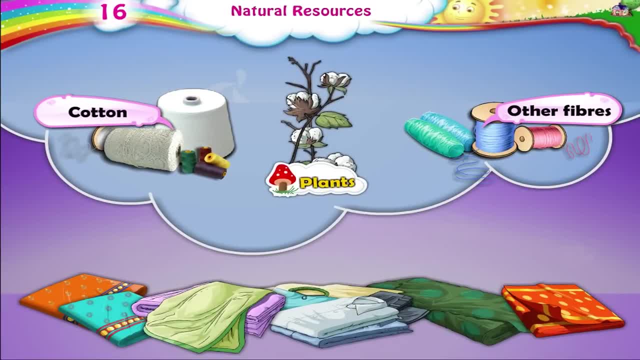 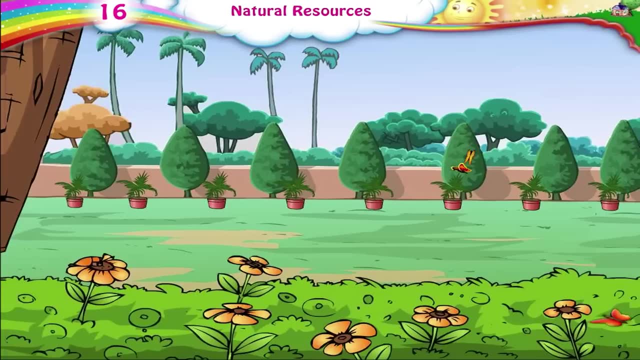 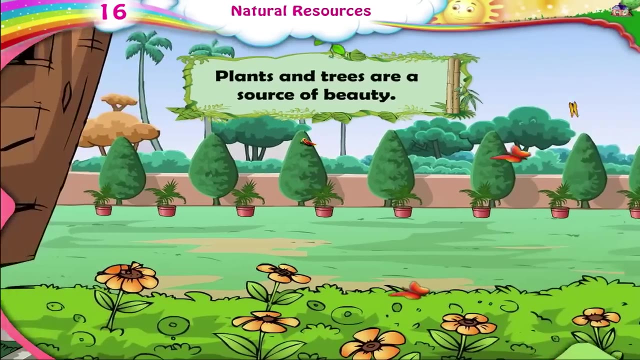 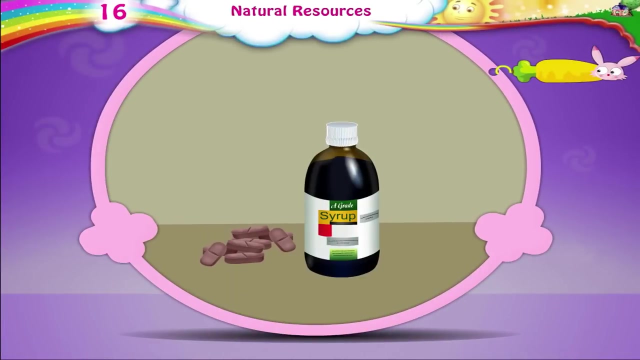 that are used to make our clothes are got from plants. This garden is so beautiful, Papa, All because of the trees, plants and flowers in it. Plants and trees are a source of beauty. That is why they are used as decorations. We also get different kinds of medicines from plants. 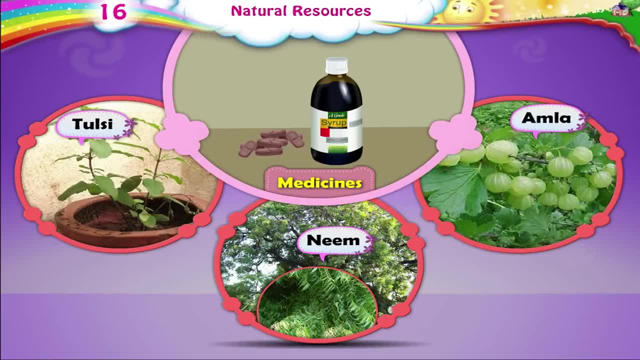 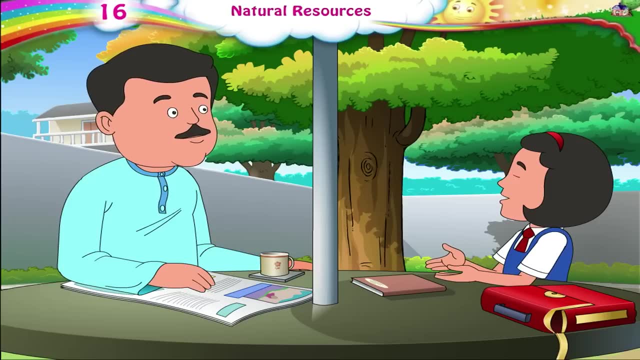 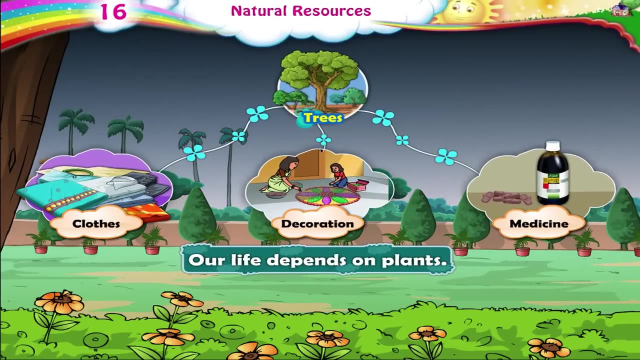 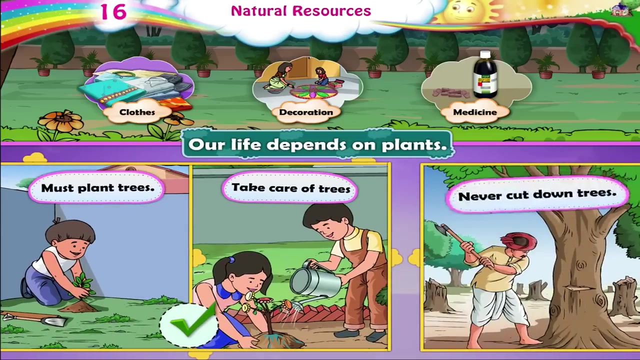 such as Tulsi, Neem and Amla Papa. fruit juices, too, are prepared from the fruits of plants. We get so many things from plants. Our life depends on plants. Therefore, we must plant trees, take care of trees and never cut down trees. 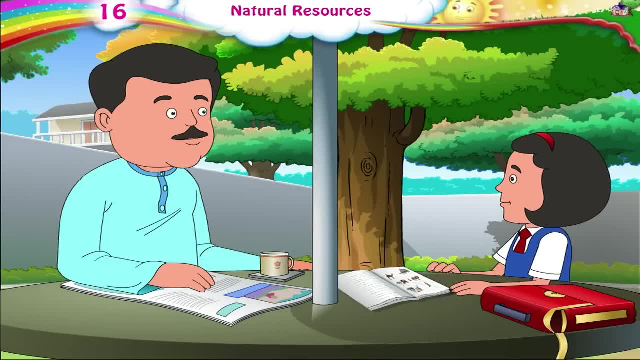 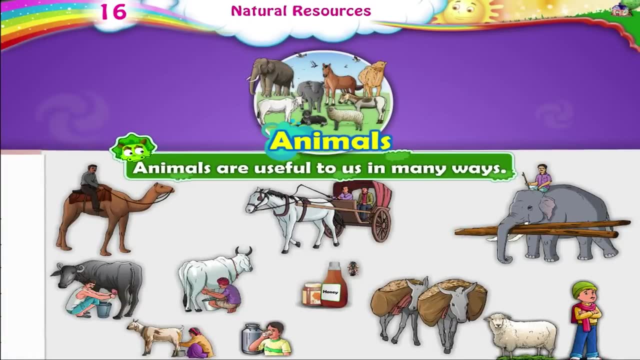 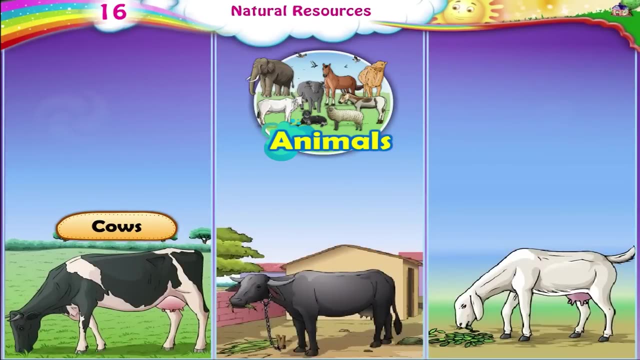 Look at all the animals. There are so many animals in this book, Papa Don't? they also help us in many ways. You are right, Rhea. Animals are useful to us in many ways. Some animals like cows, buffaloes and goats. 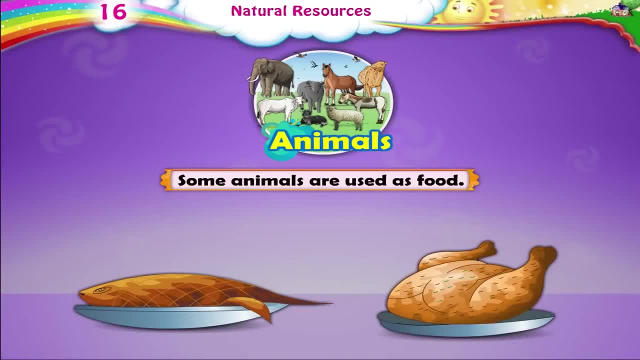 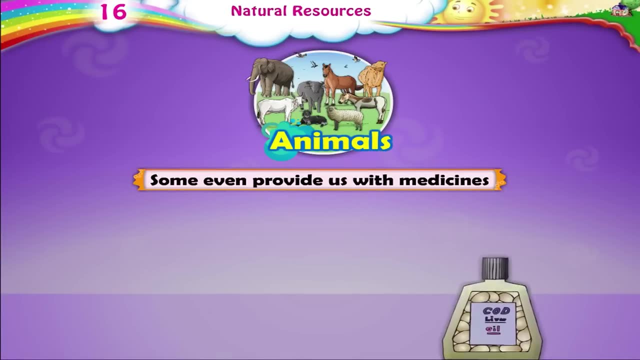 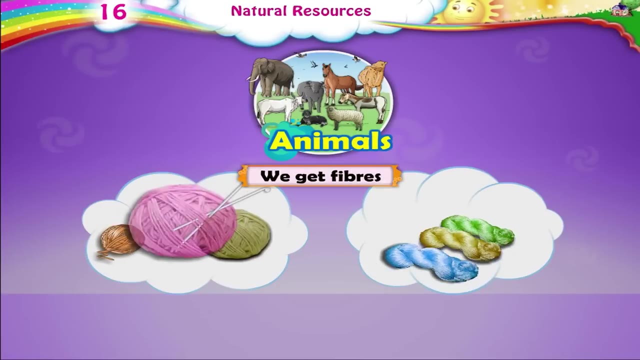 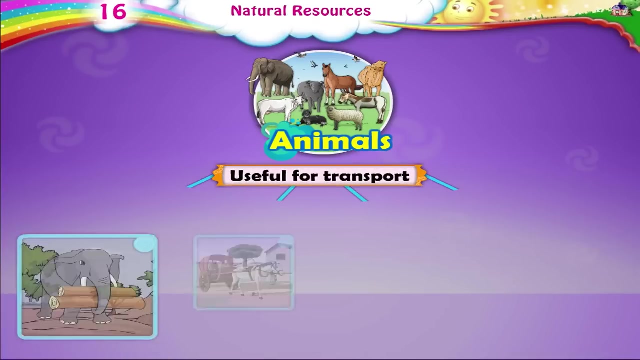 give us milk And some animals are used as food. We get honey from the honeybees. Some even provide us with medicines Like shark liver oil and cod liver oil. We get fibres like wool and silk to make our clothes. Some are useful for transport. 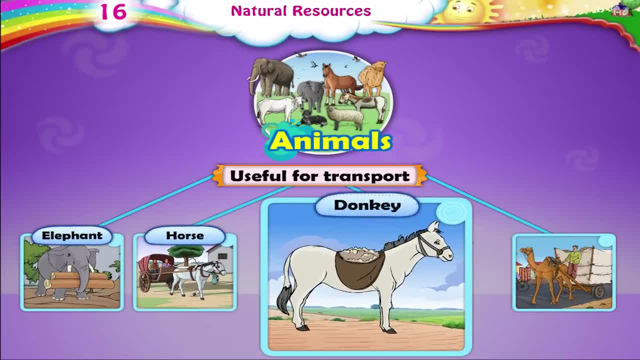 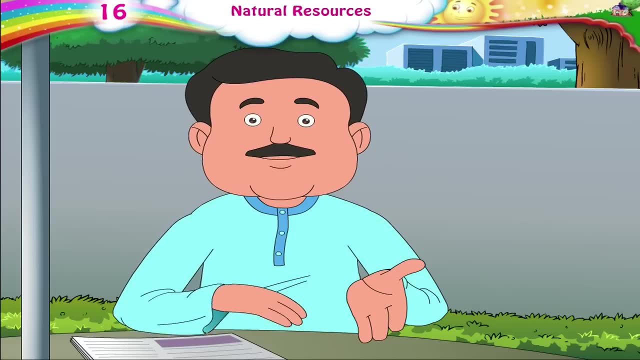 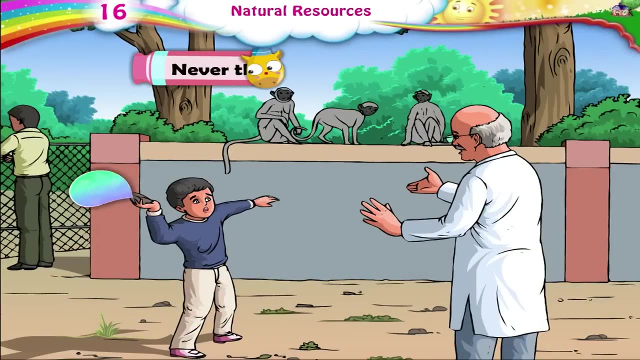 like the elephant, horse, donkey and camel. Since animals do so much for us, we must protect them. Yes, Papa, We must take care of them. Never throw stones at animals. Never throw stones at animals, Never destroy their shelters. 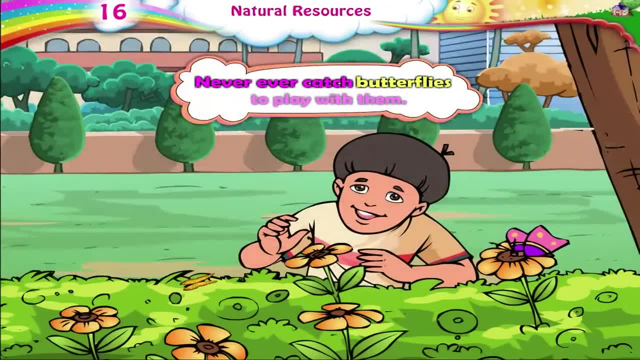 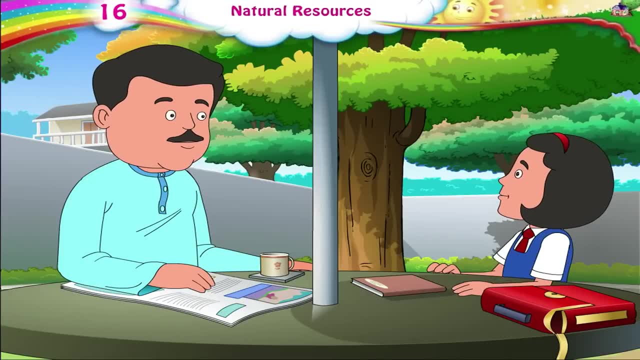 Never destroy their shelters And never, ever catch butterflies to play with them. to play with them, Papa. when we were planting trees in school, our teacher kept telling us about the importance of water and why we should not waste it, and why we should not waste it. 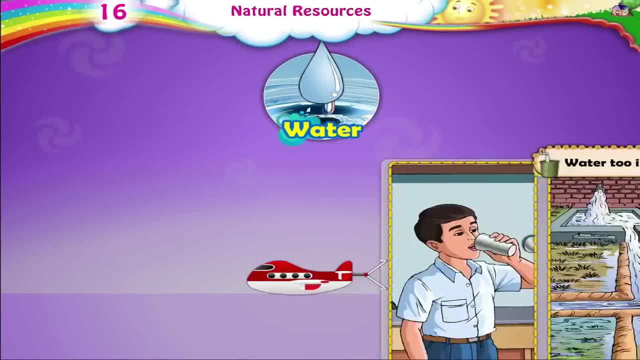 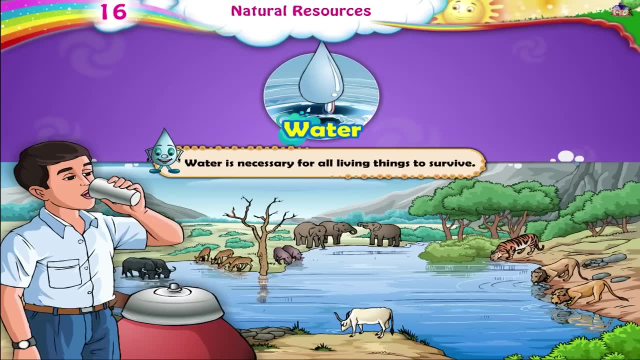 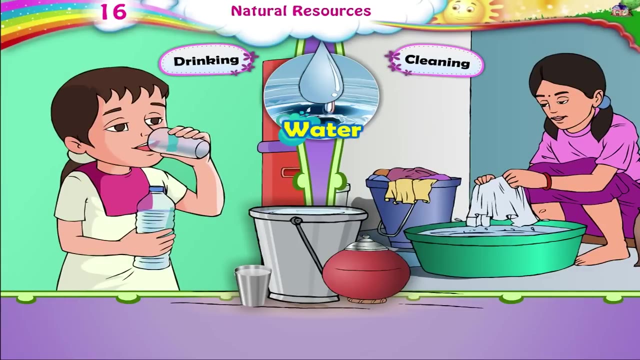 and why we should not waste it. Water, too, is an important natural resource. Water, too, is an important natural resource. Water is necessary for all living things to survive. We need water for drinking and cleaning, And for farming, producing energy and running factories. 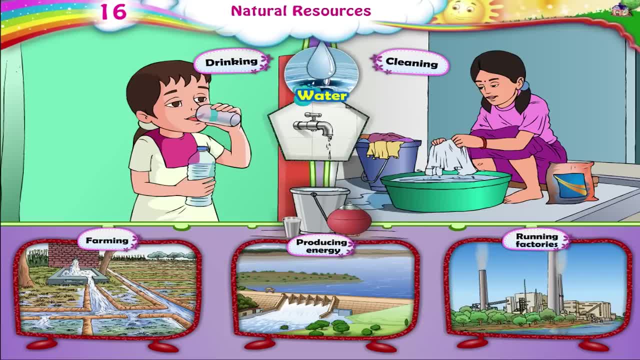 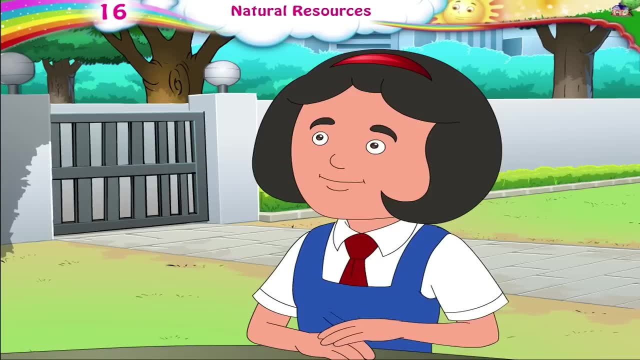 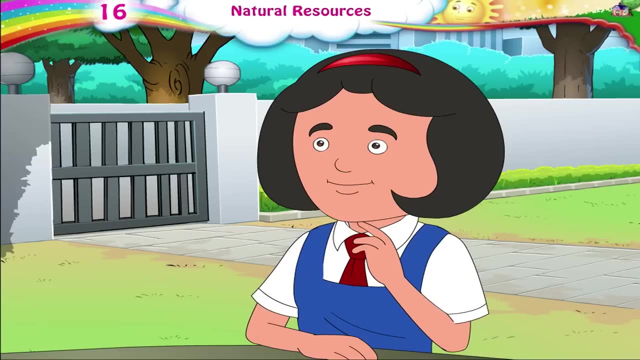 Water is needed for so many purposes, So we must use water without wasting it. What are the different ways in which we can save water? Papa, I know one for sure: Turn off the tap when the bucket is full. Yes, Rhea. 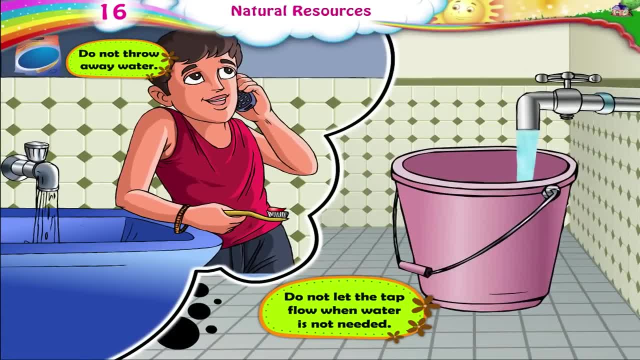 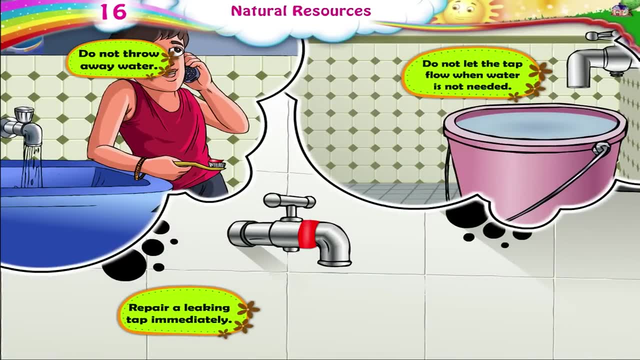 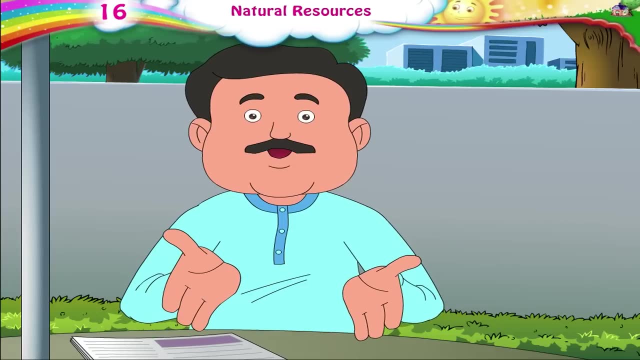 Do not throw away water, Do not let the tap flow when water is not needed, And repair a leaking tap immediately. Rhea, didn't your teacher tell you about the importance of land too? Land gives us support. It gives us soil for planting trees. 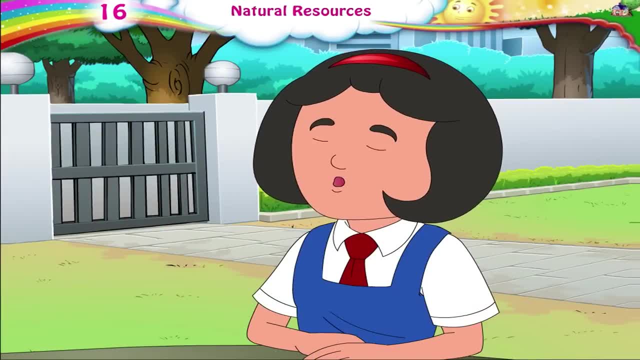 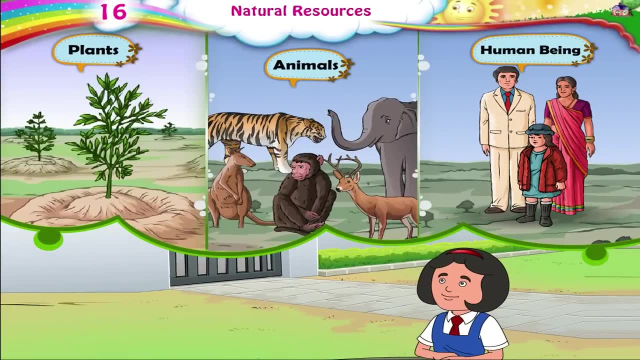 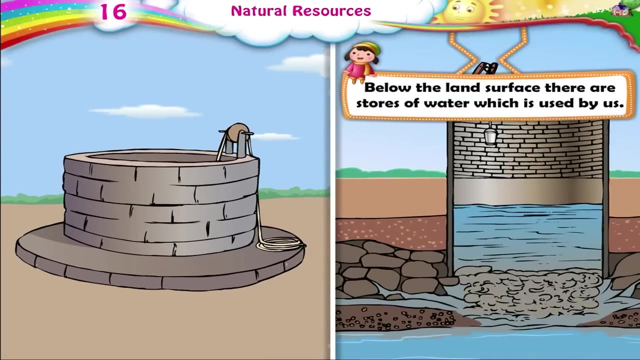 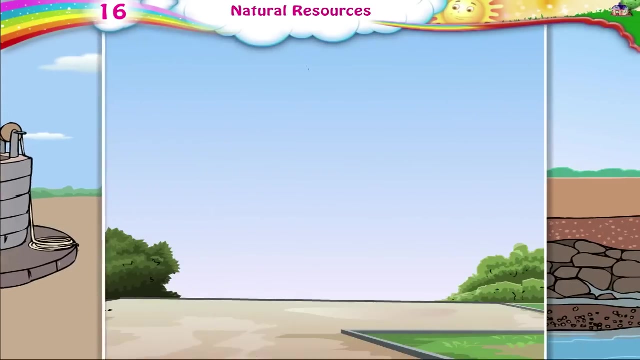 and for farming. Yes, Papa, And plants, animals and human beings all live on land. Look at that well. Where does the water come from? Below the land surface there are stores of water which is used by us Land, gives us shelter. 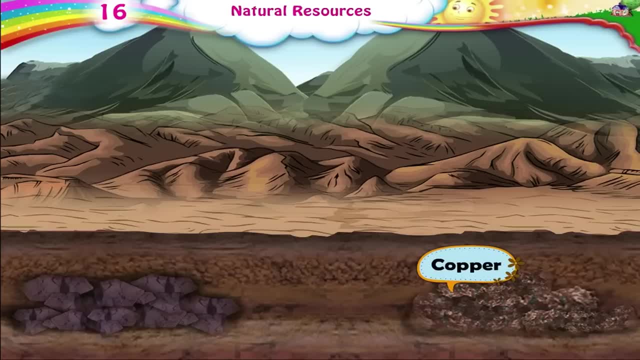 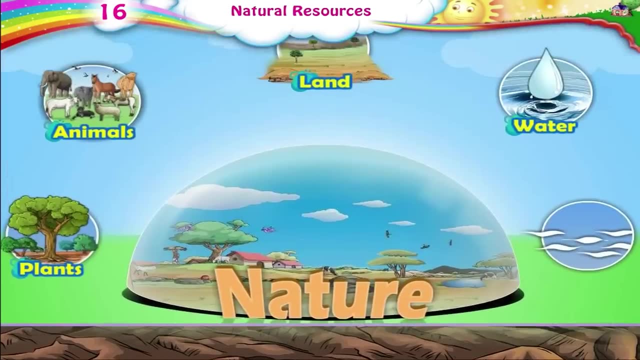 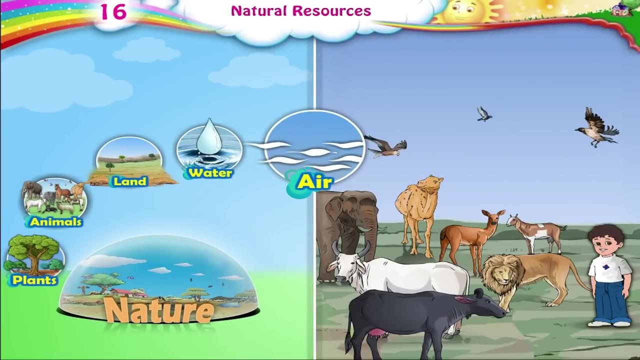 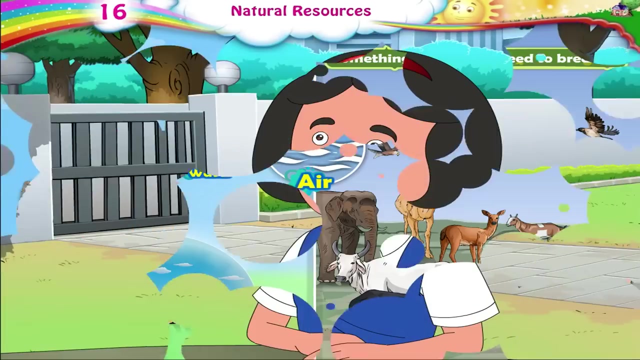 And land gives us minerals like copper and iron, which are useful in our daily life, And, of course, the last natural resource without which none of us would be alive today, Rhea, something that we all need to breathe, Is it air, Papa. 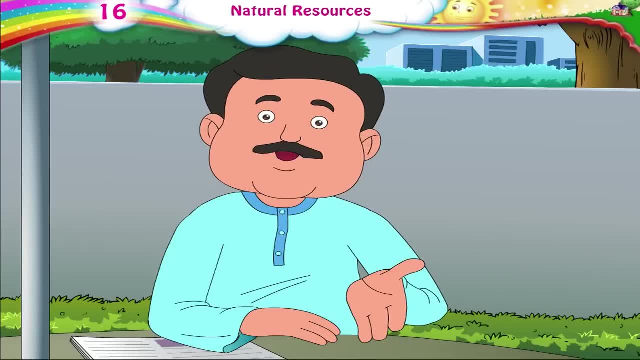 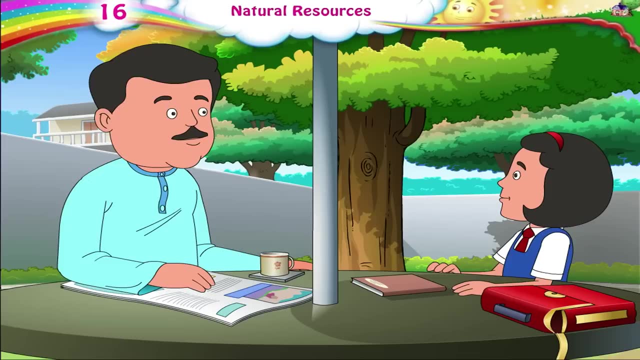 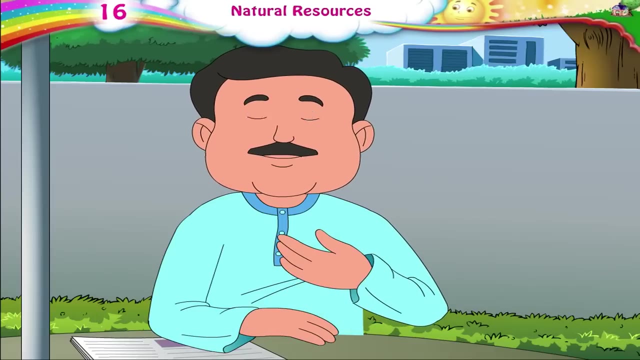 Air is all around us. How right you are, Rhea: It is air. All living things need air to survive. We cannot see air, Then how do we know it is there? When air moves, we can feel it Moving air. 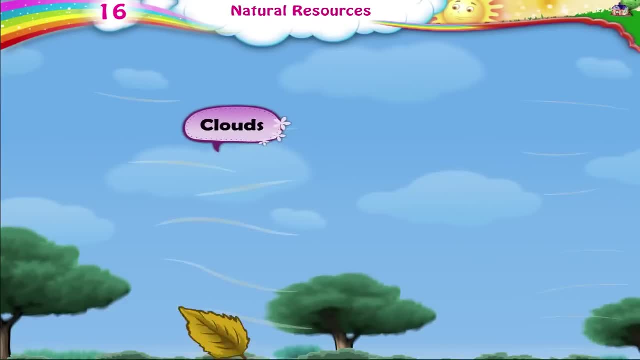 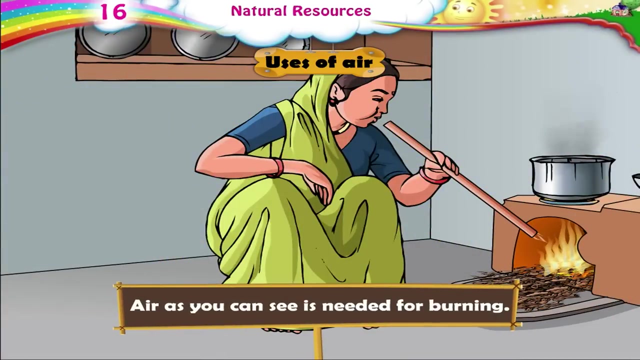 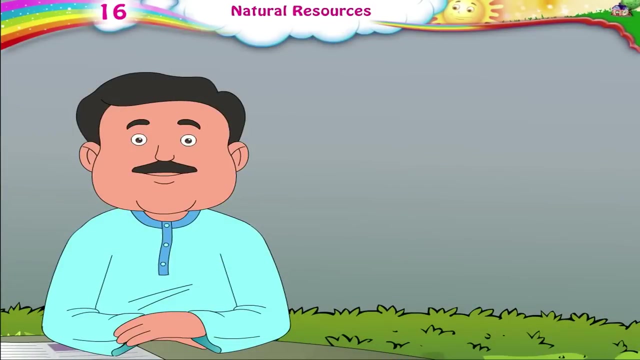 is called breeze or wind. Look at the clouds, the leaves, the kites, all moving around because of the wind. Let's talk about the different uses of air. Air, as you can see, can move boats. Yes, Air is needed for various ports. 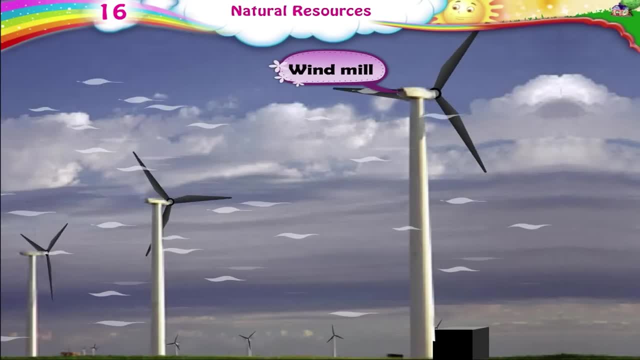 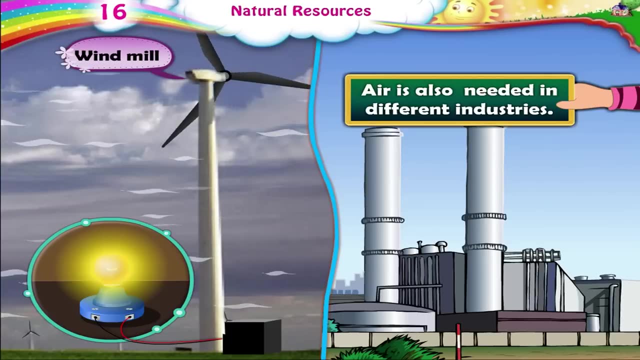 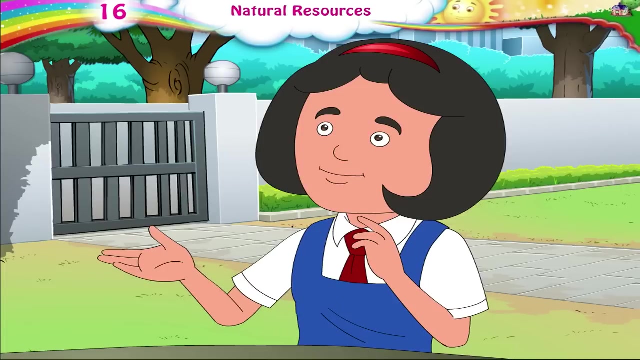 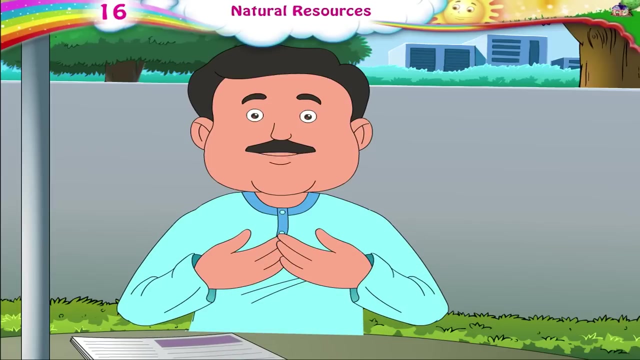 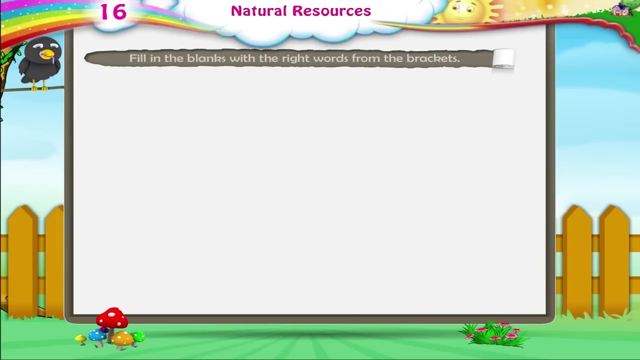 Windmills do need air to move. Air is necessary to produce energy. Air is also needed in different industries, Oh, and air is needed in transport. So you see, Rhea, we must use all our natural resources carefully. Can you fill in the blanks? 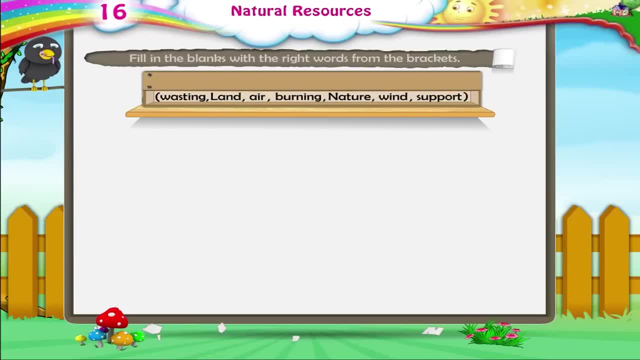 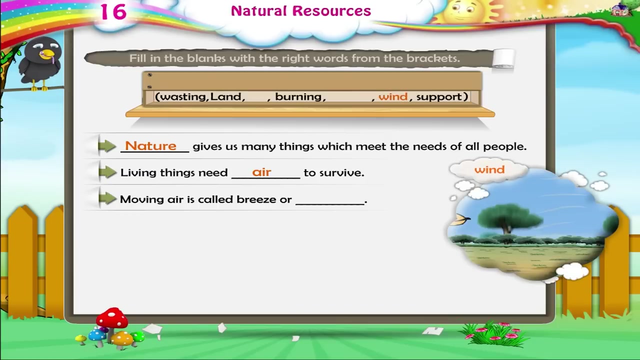 with the right words from the brackets. Dash gives us many things which meet the needs of all people. Nature, Living things need dash to survive. Air. Moving air is called breeze or dash Wind. We must use water without dash it Wasting. 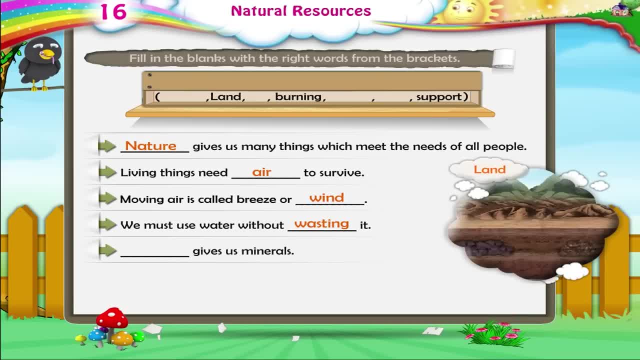 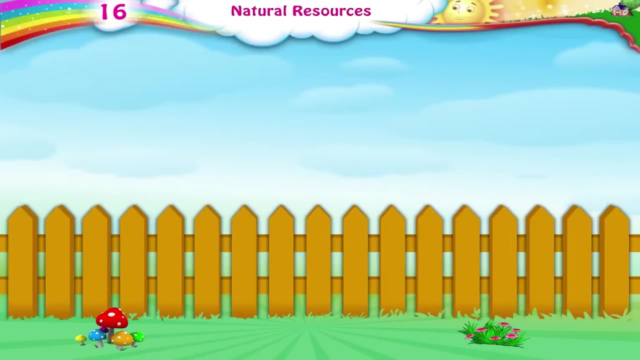 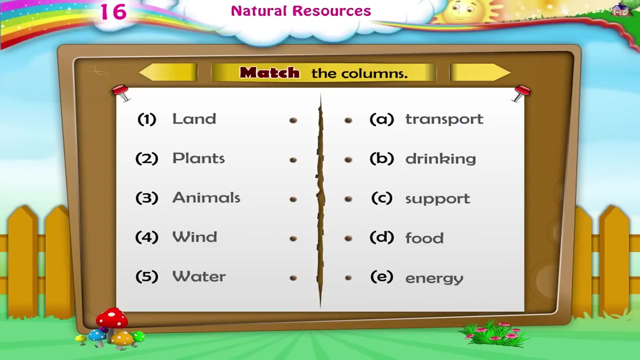 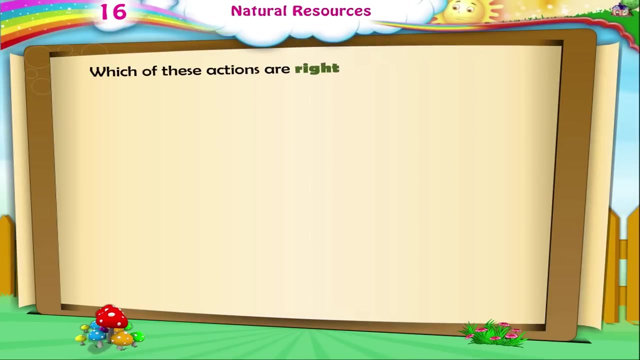 Dash gives us minerals. Land Air is necessary for dash Burning. Now can you match the columns? Land Support Plants, Food, Animals, Transport, Wind Energy, Water, Drinking. Which of these actions are right and which?